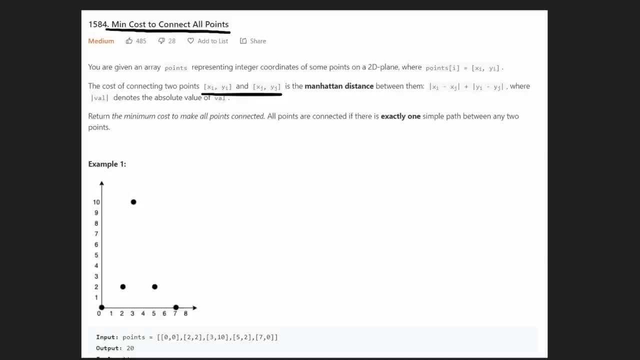 in other words the Manhattan distance, if you've heard of that term. That's pretty easy to calculate. good for us And for the entire set of points. in this case we're given five points. we want to know what's the minimum possible cost to connect all points. And they also say that 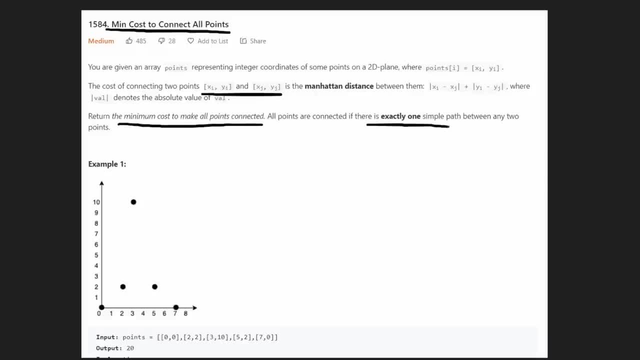 any pair of points is going to be connected by exactly one simple path. I think that information is actually redundant. just saying that we want the minimum cost to connect all points pretty much tells you this is going to be a minimum spanning tree problem. So the only question is: 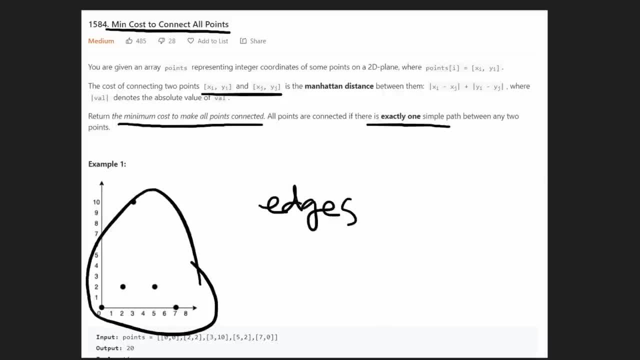 where the heck are the edges for this graph? We're only given points, right, But they do tell us pretty much what an edge is going to be right. The cost of each connection is just going to be the distance. so we have to create our edges ourselves. So basically, all possible edges. 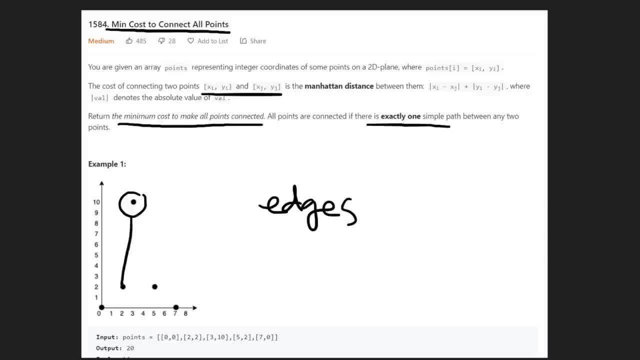 could be. you know every single point to connect it to every other point. right, That's going to be a set of edges and we can continue that. So, for example, you know this point to connect all the other points as well. So we're going to have to kind of manually create. 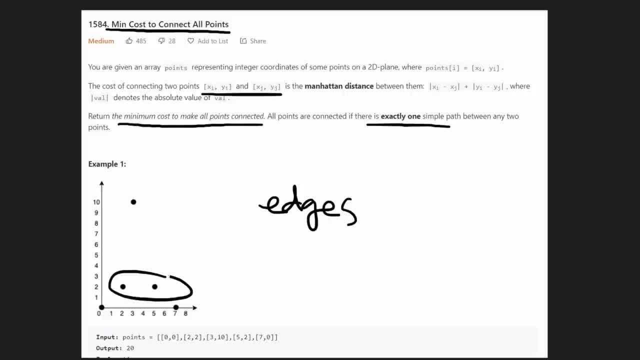 the points. So for each pair of points in the entire graph, we're just going to take the Manhattan distance between them and just call that an edge, and then, you know, have our list of edges, or basically we're going to create an adjacency list. So that is kind of like the pre-work we have. 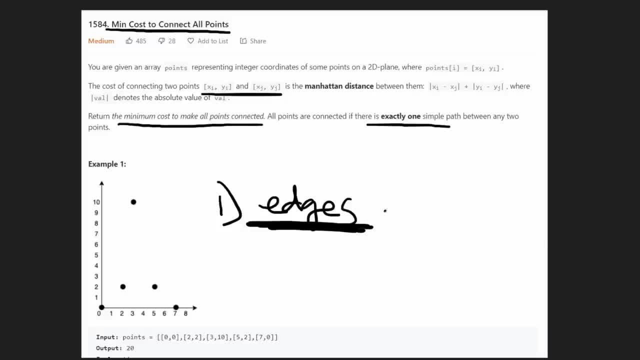 to do. That's step one in this problem: creating the edges. But as soon as you create the edges, this is literally just a problem that you can go ahead and take Prim's algorithm and just apply the textbook definition of Prim's algorithm to this problem and you will get the optimal solution. 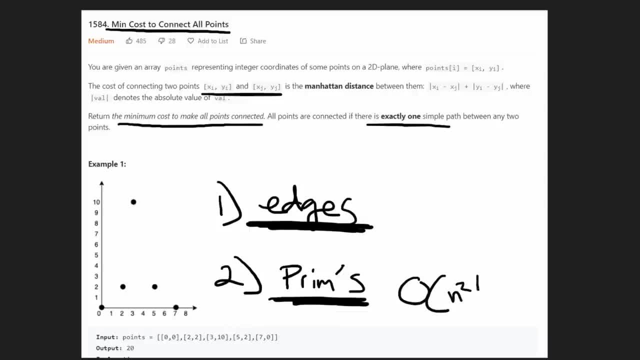 And the time complexity of that is going to be n squared. log n because n squared is going to be the number of edges we're going to have, right, Because to connect each pair of points we could potentially have n squared edges, where n is the number of points that we're given. 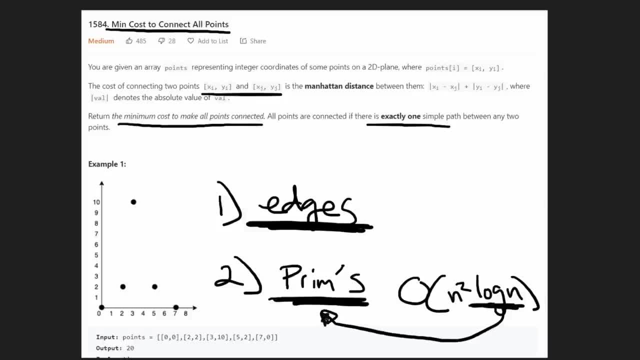 And log n is going to come from Prim's algorithm, So we're going to be using a min heap in this problem. So it's pretty similar in a way to Jijkstra's algorithm, the Jijkstra's minimum path algorithm, If you are familiar with that. 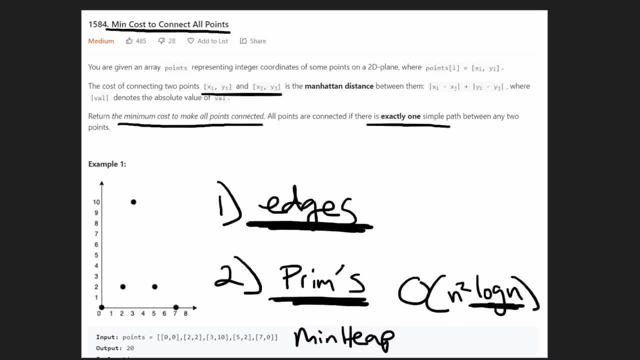 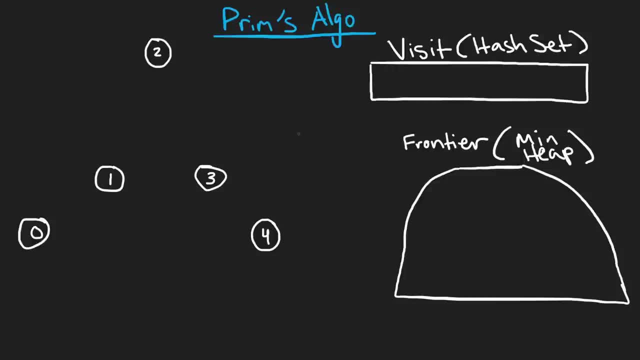 Prim's algorithm is pretty similar to that, So let's jump into it. So Prim's algorithm is an algorithm to find minimum spanning trees. So there's a few concepts you have to be familiar with to understand Prim's algorithm. Obviously, you need Prim's algorithm to solve this problem. 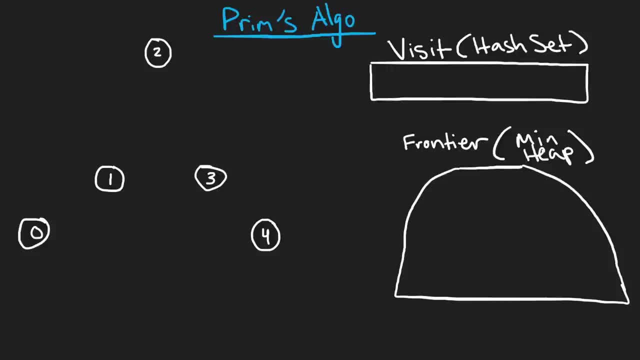 efficiently. So I'm just going to give some examples. So I'm going to give some examples of the background, in case you don't know it. So, basically, let's say you have a graph, And in this case we have a graph with five nodes or vertices right. And to connect all of these, 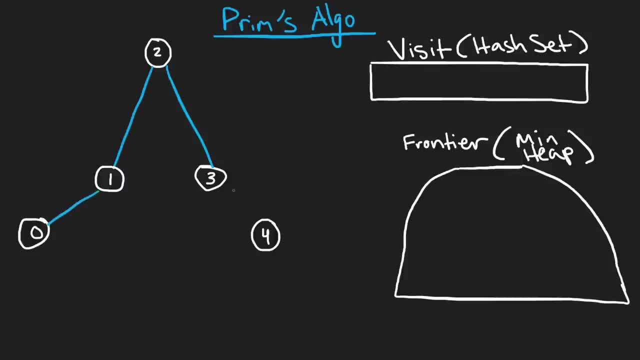 nodes together without forming a cycle. So we want every node to be connected together, but we don't want to form a cycle. How many edges is it going to take us to accomplish that? It's going to take exactly n minus one edges. So if we have five, 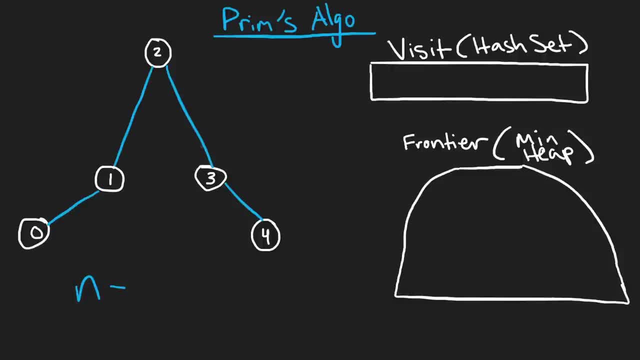 nodes. it's going to take exactly four edges to connect all of them together without creating a cycle, because take a look right now I have four edges, right. If I add another edge, that's not a duplicate. If I add an edge here, we create a cycle. If I add an edge here: 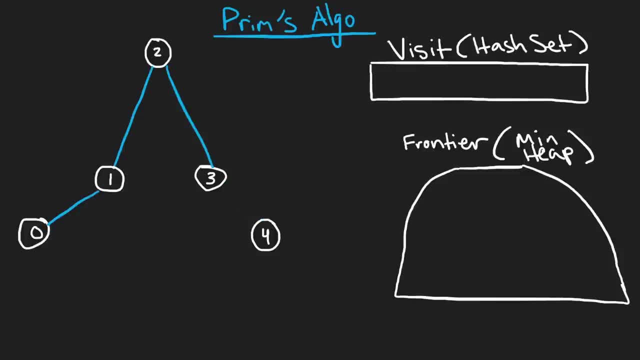 we create a cycle. If I add an edge here, we create a cycle. right, That's just kind of something you know and I think it intuitively does make sense, Because you know, if you start out with five nodes, you add one edge. Now we have four different, you know, connected components. 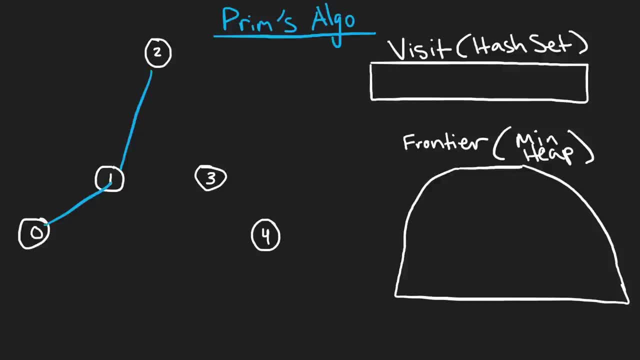 one here, one here and then a couple here. Every time you add an edge you're decreasing the total number of connected components by one. So if we start out with five nodes, we add four edges, we decrease the number of connected components by four. then we're going to be left. 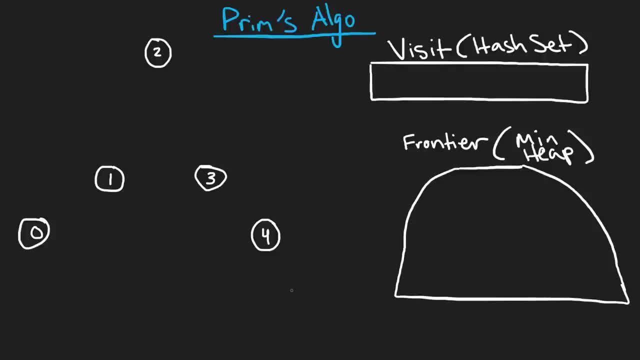 with one connected component. So if we add another edge on top of that, we're going to get a cycle. So we want to connect all of these without creating a cycle, because that's what a minimum spanning tree is. So our goal is to connect all of these with exactly four edges. but 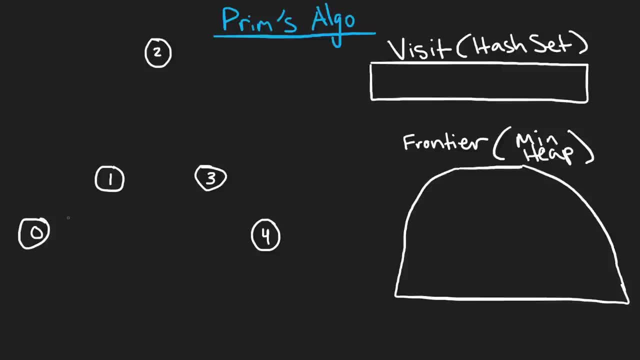 we want to minimize the total cost of the edges. Now I didn't actually draw all of the edges, all the possible edges, out. right now it would look something like this: right, Basically for every single node, it could possibly be connected to every other single node. 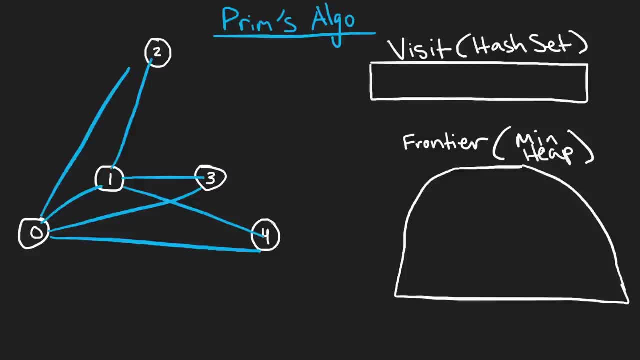 And the reason I'm not drawing it is, as you can see, it's going to get really complicated really quickly. So this is pretty much what it would look like if I drew every possible edge that could exist in this graph, And I think that's going to make it a little bit too messy. But 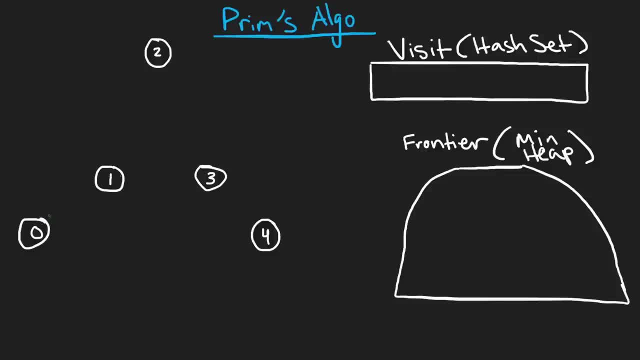 let's just assume that those edges do exist, that for any point we could possibly connect it to another point. So the way Prim's algorithm works is we can choose to start at any single node in the entire graph And then, very simple, we're just going to perform a BFS. 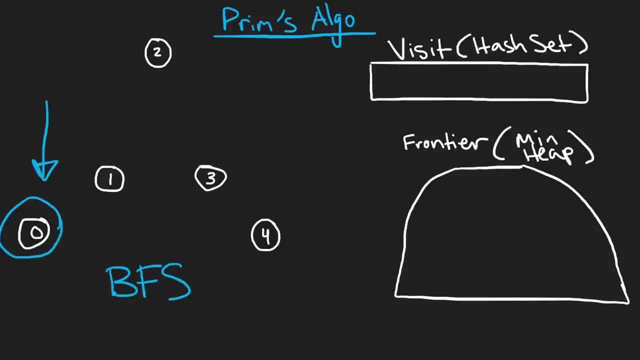 a breadth first search on that node where we are going to continuously be. for every node we're adding, we're going to have two data structures. we're going to have a visit data structure to make sure that we don't add the same node twice, Because if we add the same node twice, 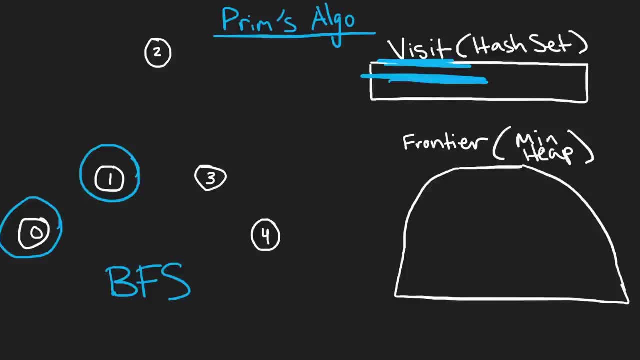 that's how you know we're going to get a cycle. we want to avoid cycles. The second data structure we're going to use is a minimum heap, which is going to keep track of our frontier, of our breadth. first search Now what is a frontier? Well, you might know that, let's say, we had a single node. So 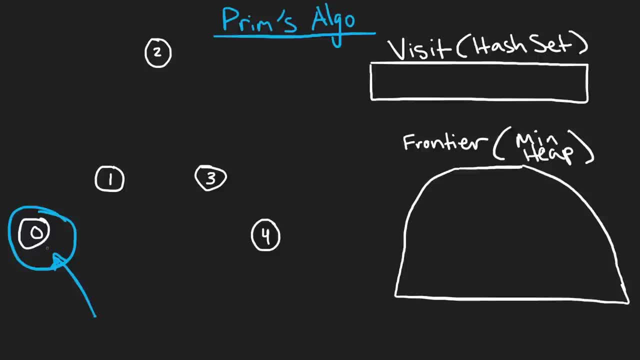 this is in our graph right. This is part of our minimum spanning tree. what's the frontier then? basically every possible node that could be added from this position, right? So initially, if we just had one node, these four nodes would be in our frontier. but we're not just going to have 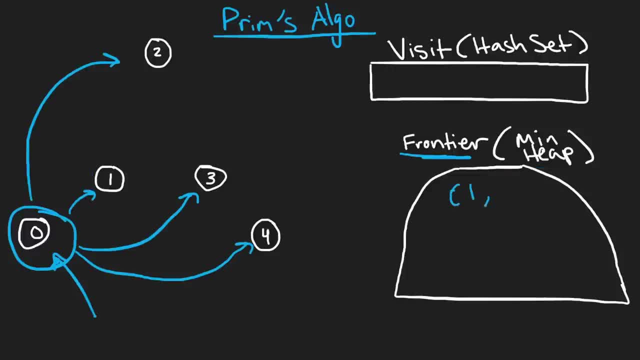 each node in the frontier. So we're going to have, you know, let's say, node one, and we're also going to add the weight of connecting node one. So let's say the weight of the edge was something like five. 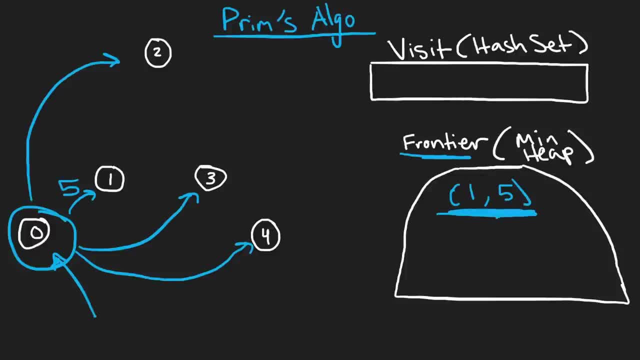 add one five in our min heap, but we're not going to add it in this order. we're going to add it in the opposite order: five, one. because when we're popping from the min heap we're going to be wanting to pop whatever node we can connect next with the minimum possible cost. so let's say we 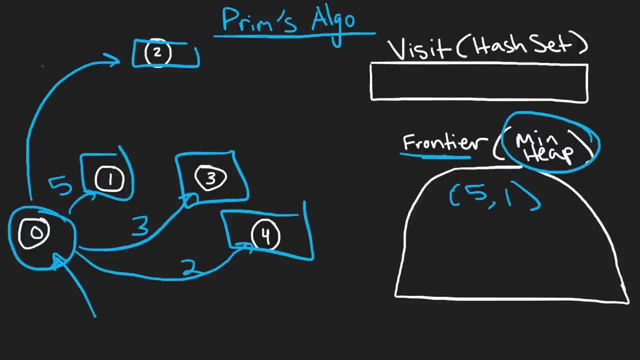 had five, you know three, two and you know up here we have a six or something. out of all these four nodes, which of them can we connect with the minimum possible cost? that's what we're going to use our min heap for. looking at it you can tell: okay, this one because it has a cost of two. so then, 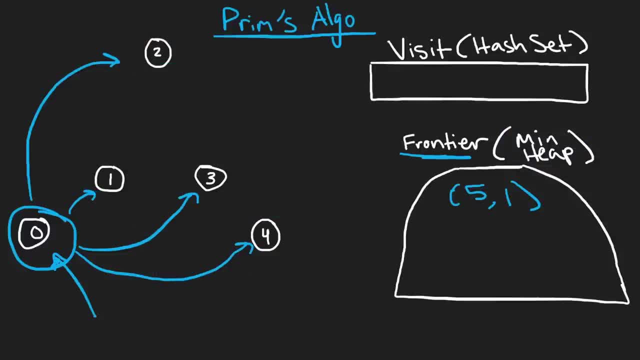 we're going to connect that that. so then, that's going to be a part of our frontier. so next, we're going to say, okay, we have two nodes a part of our frontier. next, what we're going to do is add more nodes to our frontier, even though we already had all three of these nodes. we're going to add them. 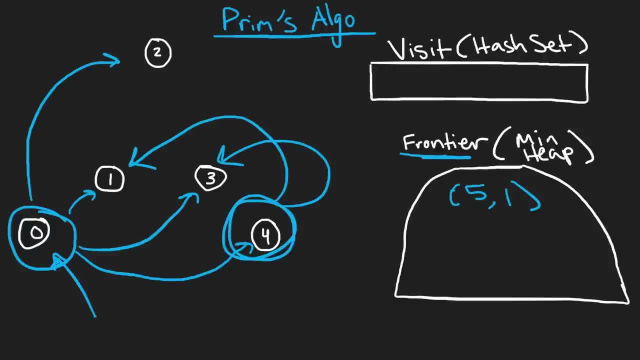 again to our frontier. because now possibly, if we're, if we're starting from node four and we're trying to connect to three, one or two, it's possible that the connection from four to three or four to two or four to one could be smaller than the connection from one to those respective nodes. so we always want to. 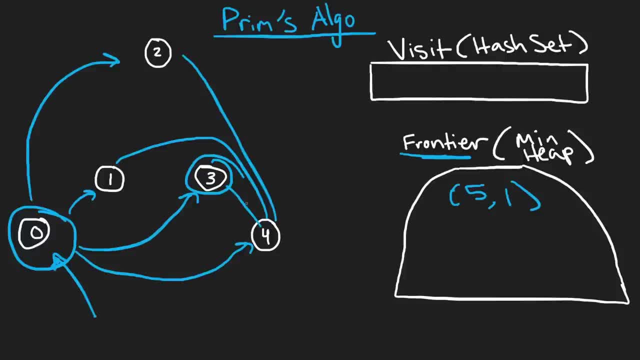 connect a node with the minimum possible cost that it takes us. if it costs less to connect it to four than to connect it to one, we're going to take the one with the smaller cost and i'm going to say that's what we're going to do. next, we're going to take the one with the 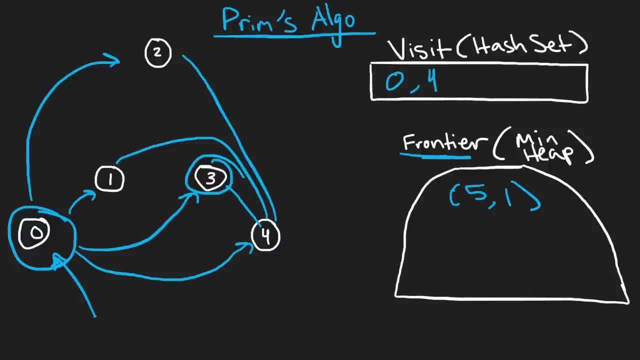 minimum possible cost. and, of course, as we visit nodes, we visit zero, we visit four. we're going to add them to our hash set so that we don't you know, starting from four, we're not going to go back to one and add one again, because that would create a loop. and how do you know that we can stop the? 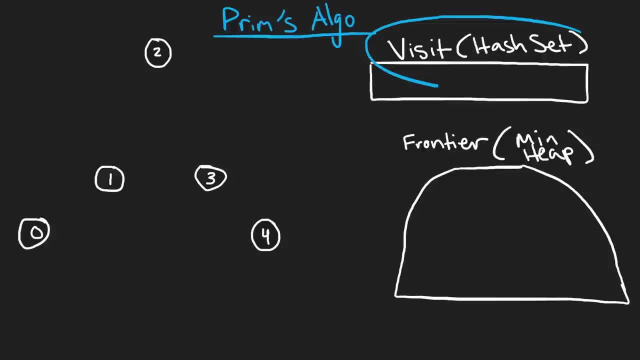 execution of prim's algorithm. well, once the length of our visit set the, the number of nodes that we've added is equal to five, which is the number of nodes that we started out with. so, with all that being said, you just have to understand how these data structures are contributing to the. 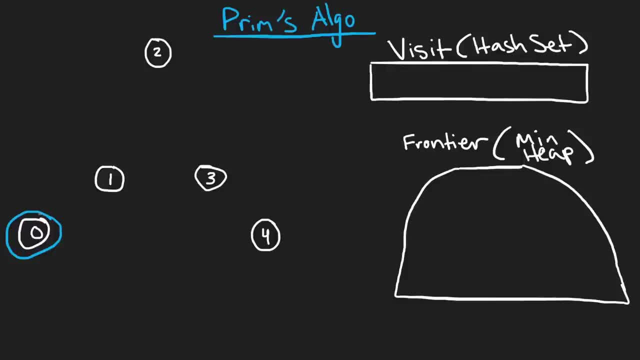 solution and then we can go ahead and walk through it. so let's start at zero. you can start at any node. you can start at three, two, four, but in this case we're going to start at zero, just because it makes sense. so when we start at zero, what we're doing is we're adding it to visit and we're adding. 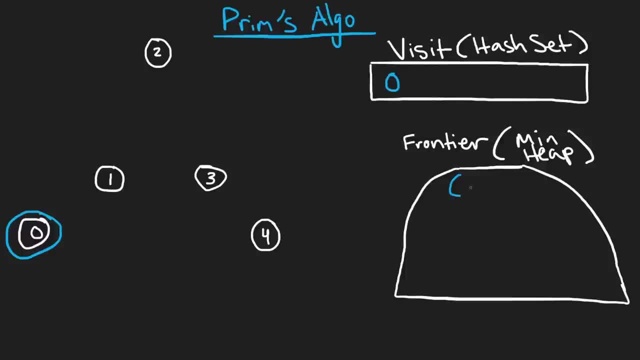 it to the frontier. so what's the cost of connecting zero? well, if we're just connecting a single node to the graph, we're not actually including any edges, so the cost is going to be zero and the node value is going to be zero. and so the way this algorithm works is, at each step, we're just going to. 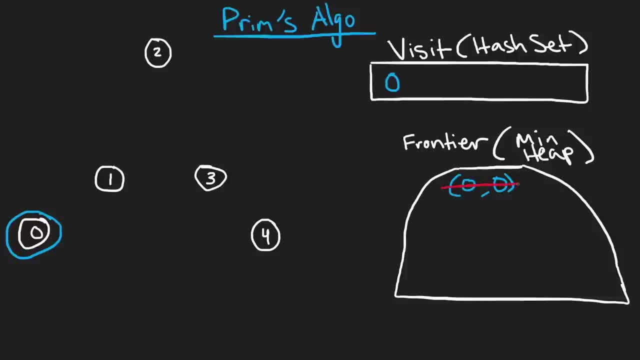 pop from the menu heap. so let's pop the first value, this, right. so the total cost so far is zero, right, we don't actually have to add any cost, and that's actually one other variable we're going to be maintaining. let me just write it down down here. so so far the cost is zero. we're going to continuously be adding. 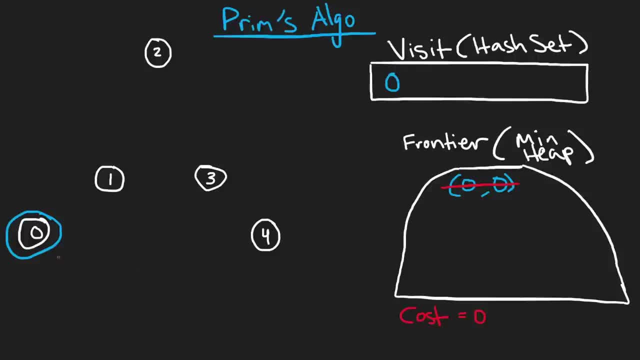 to it, though, but next for zero. we're now going to add every one of its neighbors to the frontier, and the way we're going to add it, i haven't drawn it out, but there is going to be like an adjacency for zero. of course, it could be connected to every single point in the entire graph. that's just how. 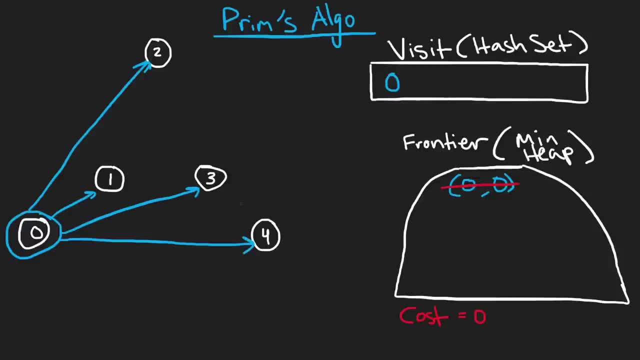 this problem is defined. now i'm not going to write the exact cost of each of these edges, because i think it's pretty obvious from the picture that this is going to be the one that's closest and the cost of connecting to that is going to be four, based on the point values that we were given in. 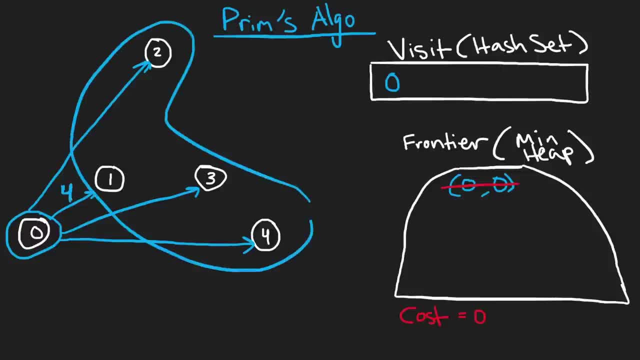 the previous picture. so out of all these four, these are going to be in our frontier. so all of these are going to be in our frontier and you can see i drew them here. i didn't specify the actual cost of two, three and four because i don't want to focus too much on that, because we know that this 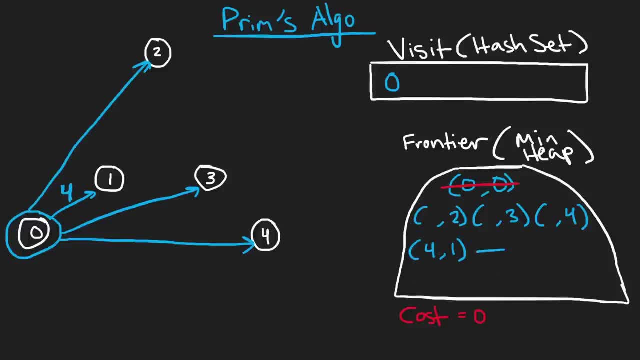 is going to be the minimum. so this is the one that we care about right now, because we already can tell from the picture that it's the smallest, and so that's the step right. so you take the entire frontier, add it to the min heap. next step: we're just going to repeat the same thing that we just 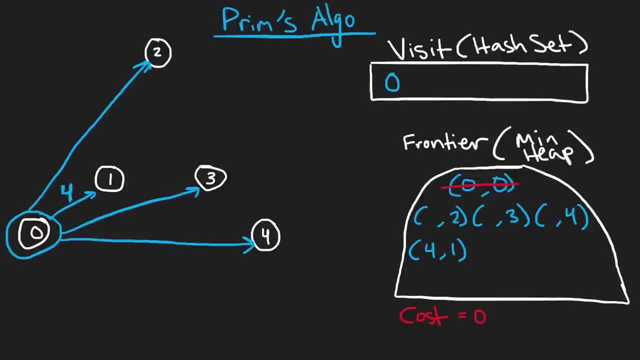 did. we're going to take a look at our frontier, pop the minimum from it. we know that this is the minimum, so pop it. when you pop a node, we have to add it to visited. so we popped the one node, right? and so we're going to add it to visit. and the cost of that one was four, right? so let's just add. 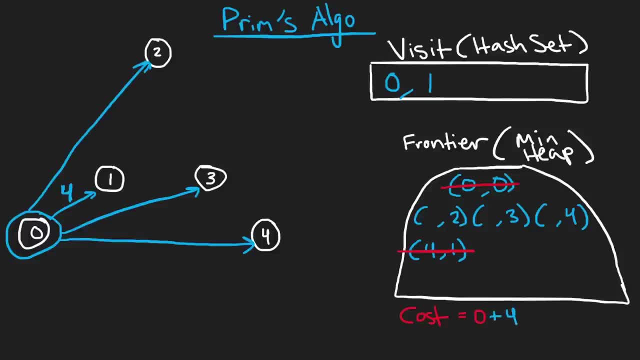 four to our total cost so far, and since this one was popped, let me just draw that. that is definitely going to be an edge inside of our minimum spanning tree. so now we are at one, and now we're going to add every adjacent node or every neighbor of this to our frontier as well. so you can see that that 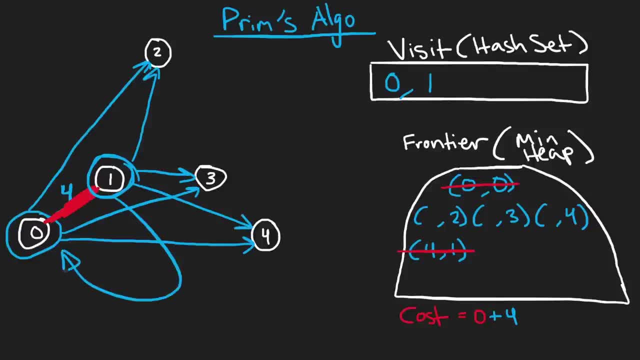 this is kind of what the graph is going to look like. we're not going to add one to our frontier because it's actually already been visited, but we are going to add two, three and four to our frontier. now notice: they already exist in our frontier, right? so we're going to be adding them multiple times. that's kind of how the n squared. 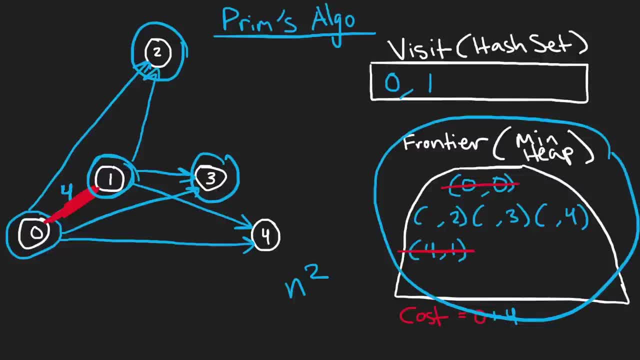 is going to come from right. we could possibly add n squared nodes to this min heap, because we're going to be adding it for every possible edge that exists in our graph and every time we pop from the min heap it's going to be log n. so basically the time complexity is n squared. 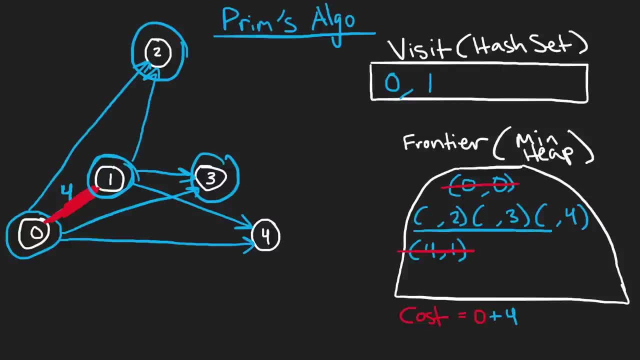 multiplied by log n. so i'm not going to redraw all three of these nodes, but you can assume that, yes, there could be duplicates of them inside of our min heap. now, looking at one, which node is the closest to it? now, of course, three is the closest node to our entire. 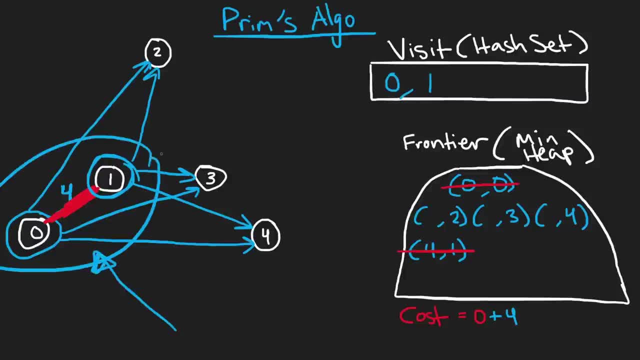 graph. this is our entire graph. right, we have two nodes, right? what's the closest node that we can add to this graph? right, we could add it anywhere. we could say, okay, this is going to be connected to zero, right, or three is going to be connected to zero, or three is going to be connected to one. 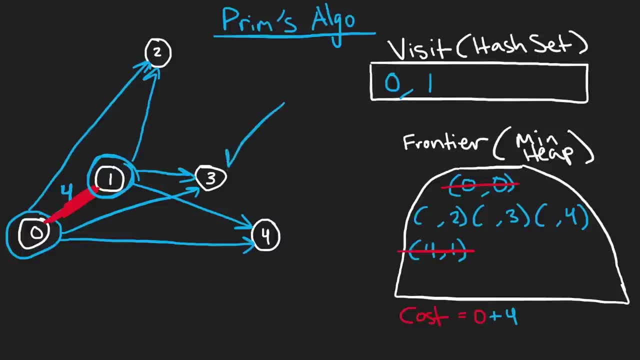 we could add any node, but we know just by looking at the picture that this is what's the closest is, and i'll just tell you: okay, for that node 3, the cost is going to be 3.. so now we continue another iteration of our loop. let's pop the minimum from the frontier. this is going to be the minimum 3. 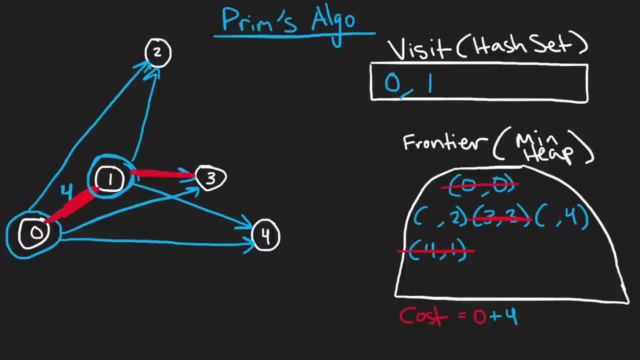 has been popped, so let's add an edge connecting it to our graph. so so far this is what our graph looks like. since we popped three, add it to visit and let's add the cost of it. so 3 was the cost of adding node 3, so total our cost is going to be 7 so far. so now 3 has been visited. 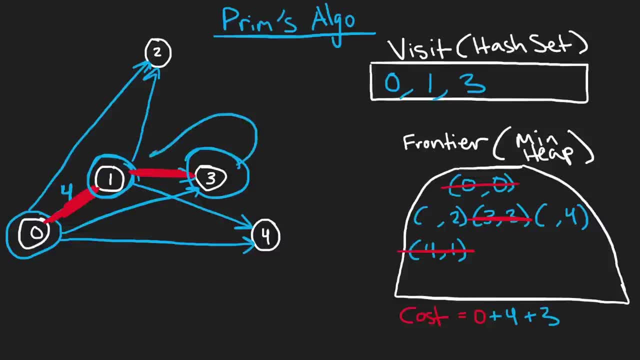 frontier. of the neighbors of three, of course, one and zero have already been visited, so we're just focusing on two and four. we're going to add those to our frontier. they're already in our frontier, but, yes, we're going to be ending up adding duplicates to the frontier, right? so i'm not. 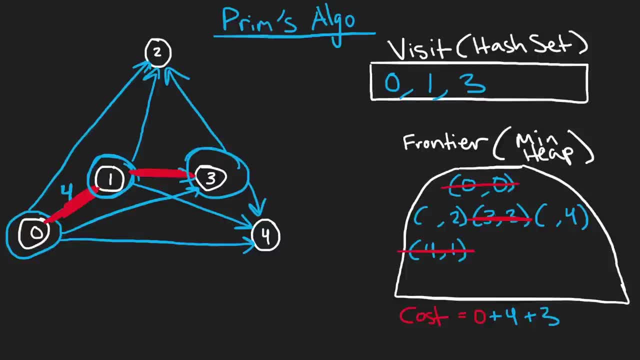 going to, you know, actually focus too much on the drawing, but there could be multiples of these in the frontier. and now, well, which of these edges that are in our frontier, or the nodes in our frontier, what's the minimum cost that we could pop? i'm just going to tell you that, for the cost, 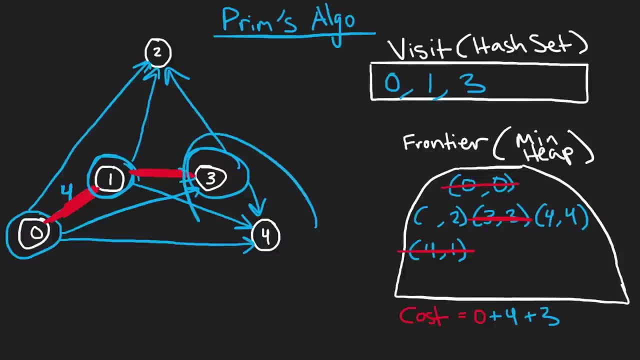 of node four. it's going to be four and it's going to be this right, you can tell by the picture. that's pretty obvious. this is going to be the shortest way to include the node four, so let's pop this node, add it to the edges list, so one or three and four are going to be connected and the 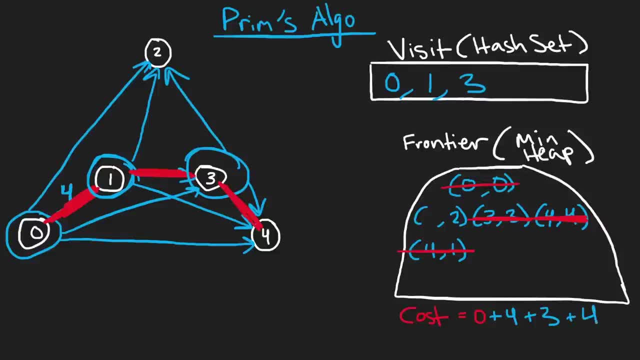 cost of that one was four. so let's add four, and let's add it to the visit now, just so you know that. let's say we did end up popping the same node multiple times because technically that's possible. right, we pop one, four, but we still have a four remaining in the frontier. so we, what if we? 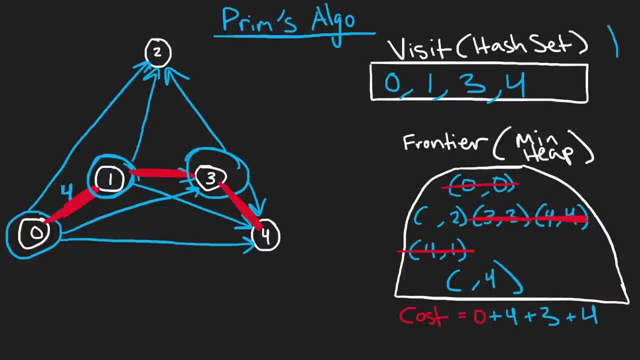 popped four again. what would we do? well, we would actually see that. okay, let's take a look at our visit. well, four has already been visited, right, so there's no need to add this to visit again, and there's no need to add the frontier of that again, and there's no need to take the cost of that. and 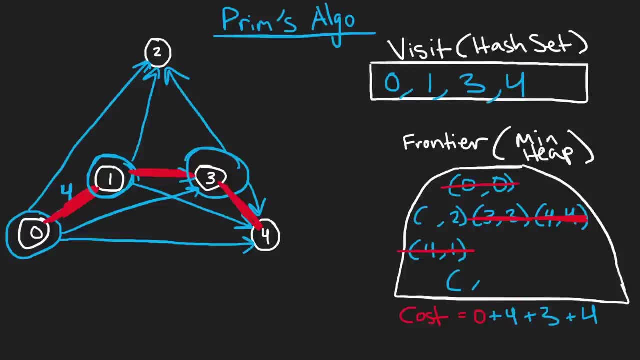 add it to our total cost, because four was already connected to the graph. don't want to, you know, add a redundant cost, okay, but so now you can see that four has been added to our graph. now what's the remaining neighbors of four? of course these three nodes have already. 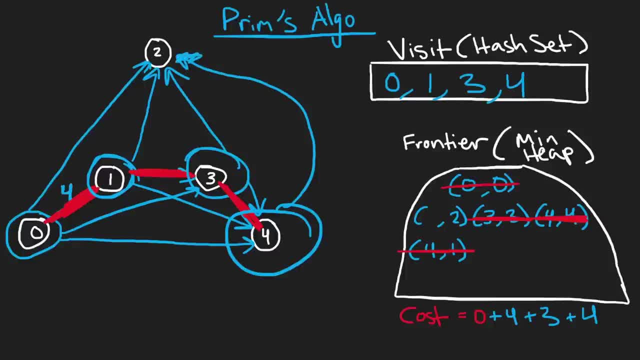 been visited, so the only edge we could possibly add that would be useful would be this to there. but you can see that that's a pretty long path, right? surely we have a shorter path in our graph to the two node? so so you can see four of them are already connected. we just need to connect one last. 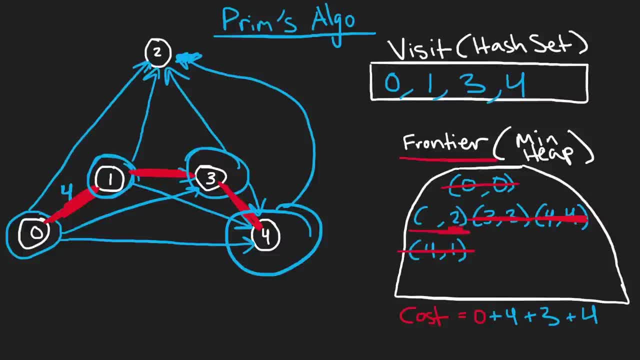 one, so let's pop from our frontier again. this is going to be, obviously, two is going to be the one exactly is going to be the cost of it. well, i'll just tell you. the cost is going to be nine, and which edge is it going to be? well, by looking at the picture, we'd probably think one of these two. 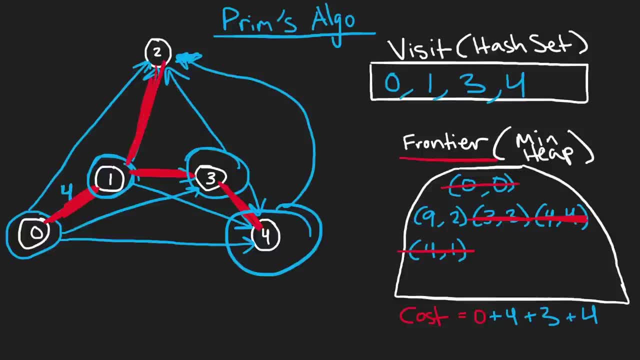 is going to be connected to two, either like this or like this, and i'll tell you that the paths are actually not of equal length. if they were equal length, it wouldn't really matter what which one we chose, right it would. it would lead to the same cost anyway. but in this case, i'll tell you this is: 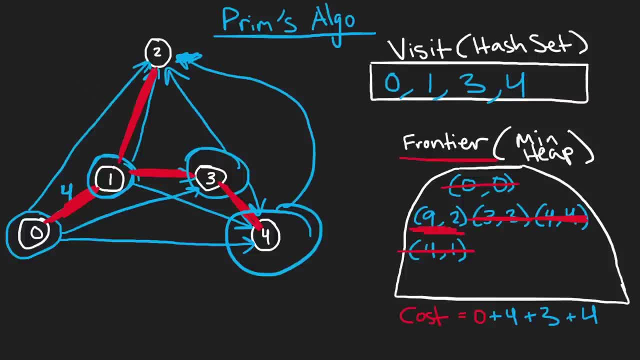 the shorter one. so- and yes, the cost of that is going to be nine, so we can pop this, so we can say two has now been added, two has been visited now. it wasn't previously visited, but now it's visited and the cost of adding it was nine. so the total cost that we ended up getting was 20. 20 was the. 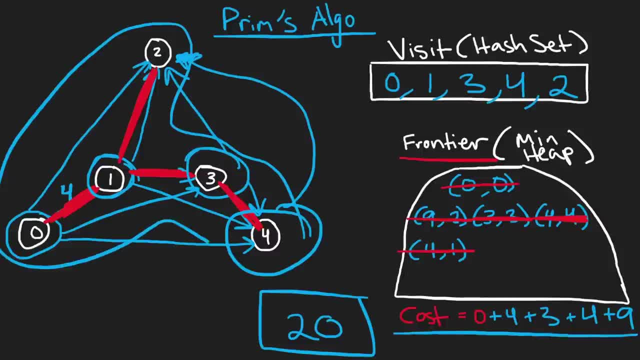 total cost. and now we know we're done because every node in our graph has been connected. you can tell by the red edges. all of the nodes are connected. we added four edges and we visited every single of the five nodes. so the algorithm- prim's algorithm- is just that simple. i mean it's. 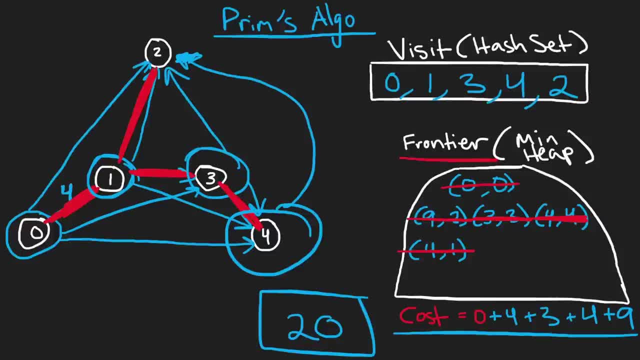 not really simple until you've actually done it a few times, you've practiced it and learned these concepts of visit min heap, and now we're actually going to jump into the code. it's about 20 to 30 lines, okay, so let's write it out and, like i said so, the first thing we're going to be doing, 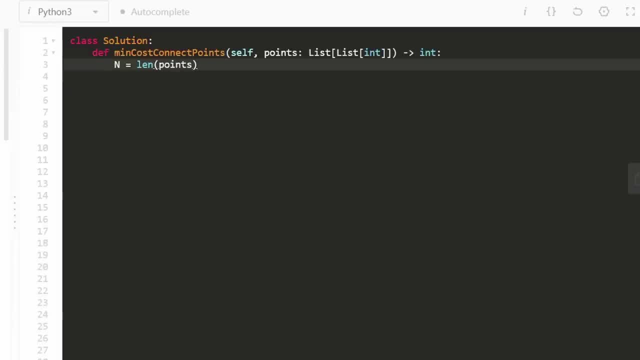 is actually creating the adjacency list, because that's not given to us. we're just given a list of points. so i'm going to get the number of points we have and then i'm going to start creating that adjacency list. so and basically i'm going to refer to each point in our list. 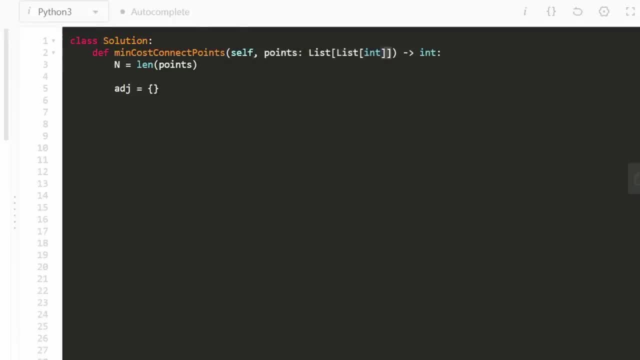 basically the index of that point. so the first point in our points list is going to be point zero, the next one is going to be point one, etc, etc. so we can just say for i in range of the number of points we have, so for i, in range of n, the number of points we're basically going to take. 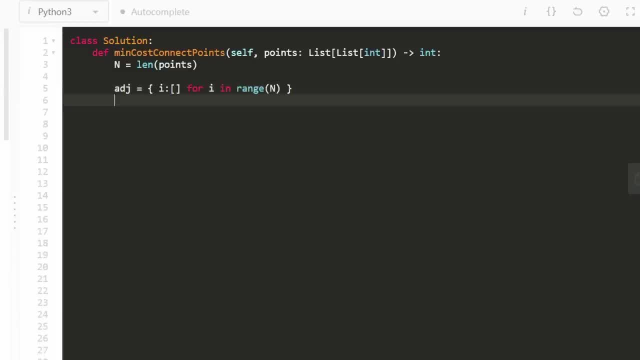 each point i map it to a empty list. so far, now we're actually going to build out that list. so for i in range of n. so for every single point we want to compare it to every other point in the graph. so for j in range i plus one all the way to n, so we don't 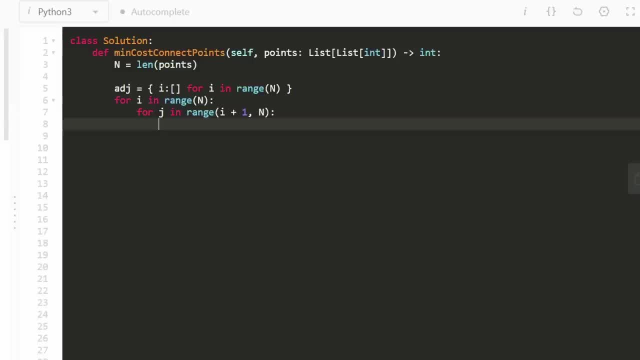 want to compare each point to itself, we just want to compare it to every other point in the entire graph, and when we do that, we want to get the coordinates. so for the point at i, we're just going to get the x and y coordinates. so points at index i, and we're going to do the exact same thing. 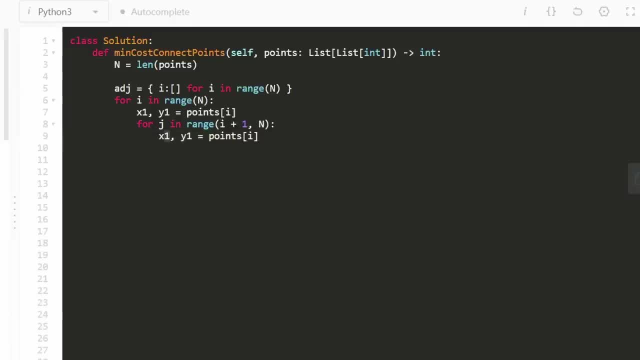 for the point at index j, inside of our loop we're going to get each point that we're comparing it to and then we're just going to take the distance, the manhattan distance, between them, and we can get that by taking the absolute value of x1 minus x2, the absolute value. 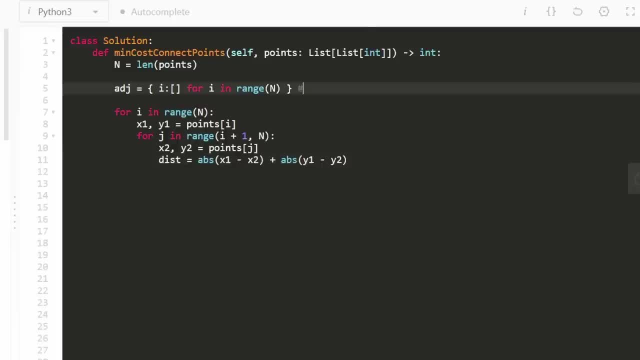 of y1 minus y2, and so i'm going to just comment up above that, for each node work, we're mapping it to a list of points and for each point we're basically going to have the cost and the node or the neighbor. each neighbor is going to be a pair, right? so each edge is basically 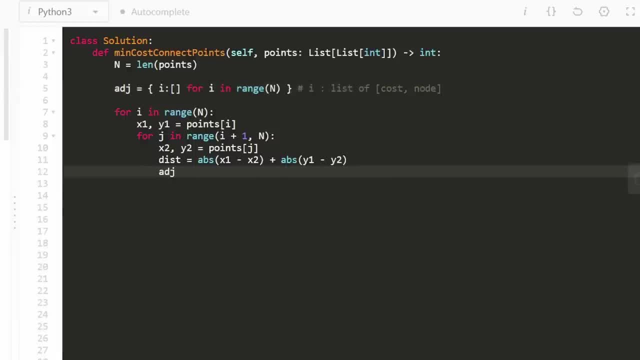 a weighted edge, don't forget about that. so we're going to say adjacency, for i append to it the cost or the distance right and the node itself, which is node j, and we're going to do the exact opposite, because technically these are undirected edges. they go both ways. so let's just do the exact. 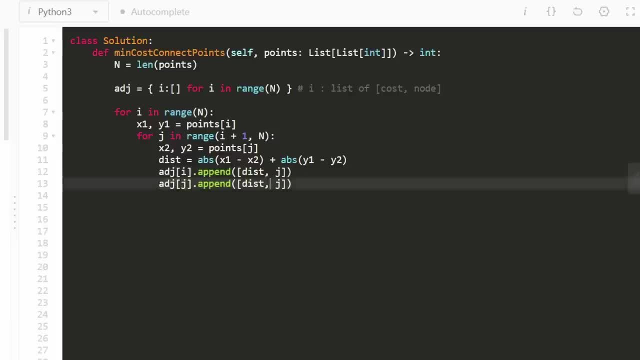 opposite. so adjacency of j: append to it the distance- same distance, but instead we're appending i, because that's its neighbor. so this is how you build that adjacency. listen, technically we could actually not have that adjacency list. we could actually not have that adjacency list if we just 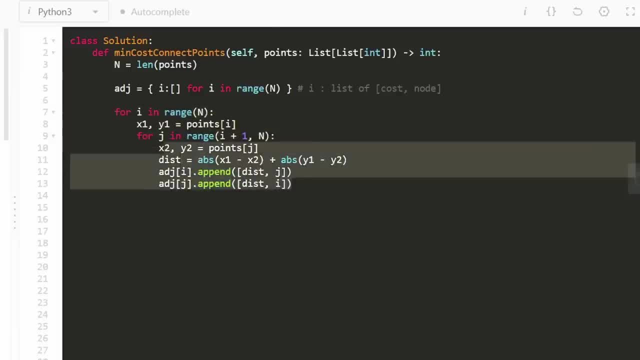 have to write this for loop out. we could actually, you know, compute these calculations while we are running prim's algorithm, but the reason i'm doing it before is just to give a clear distinction. this is the edge portion. this is like the extra portion of this problem. the following part is: 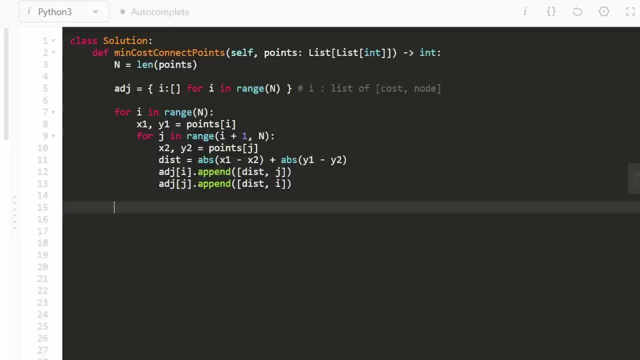 literally just an exact implementation of prim's algorithm. nothing fancy. so let's define our variables. we're going to have a result, which is, of course, going to be the total cost. initially it's going to be zero. we're also going to have a visit set, so it's going to tell us the, the 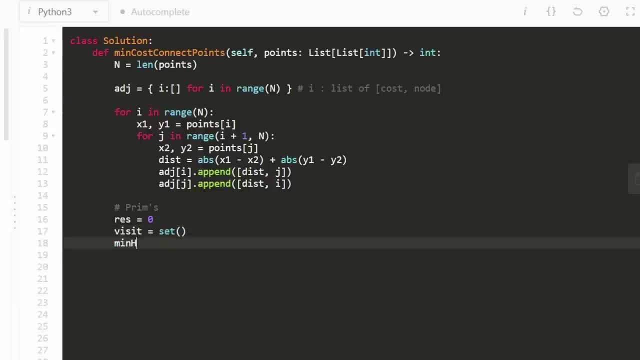 the points that have already been visited. we're also going to have a min heap, which is initially not going to be empty. we're going to be starting at point zero and the cost of it is also going to be zero. so let me just put in a comment that each pair is going to be the cost and the point cost. 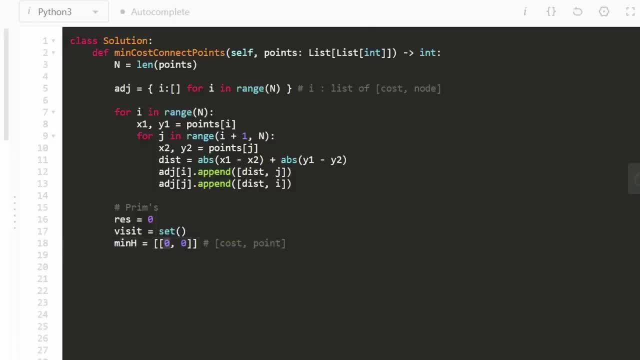 goes first. the order is important because that's what the min heap is going to be minimizing it based on, and so now we're actually going to do the loop and remember, we're going to keep going while the length of visit is less than the total number of points, which is n, and our 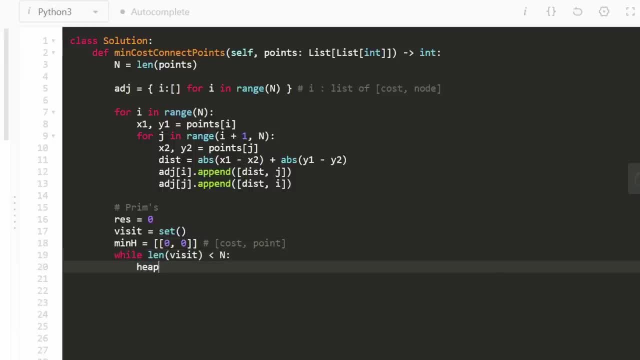 each iteration we're going to be popping from the min heap. in python we can say heap q, dot, heap pop, and from it we'll get a pair of values. okay, we have to specify which heap we're popping from- min heap, min h- and we're going to get a pair of values: the- we can call it cost, and the point- let's call 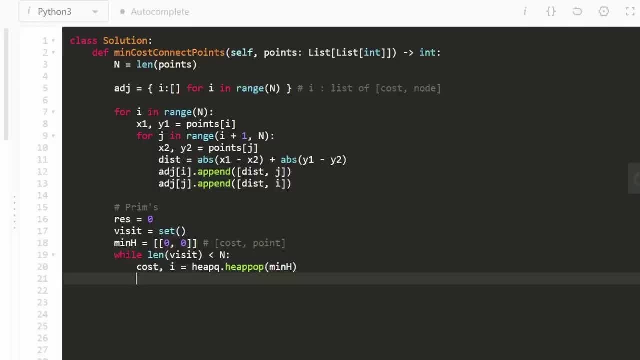 it i, and remember we are adding duplicates to our min heap, so if we popped it this could have already been visited. so let's just check. if i is in visit, then we're just going to skip this iteration of the loop. we don't want to have to process the loop we're going to have to process. 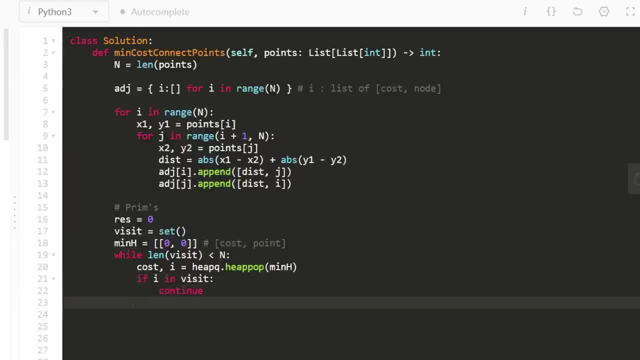 this same node that's already been popped before. but if it hasn't been popped, then we're going to take the cost of it, add it to the result. so we're adding this fresh new node that we haven't visited yet and we're also going to add it to visit now to make sure that it never gets visited again. 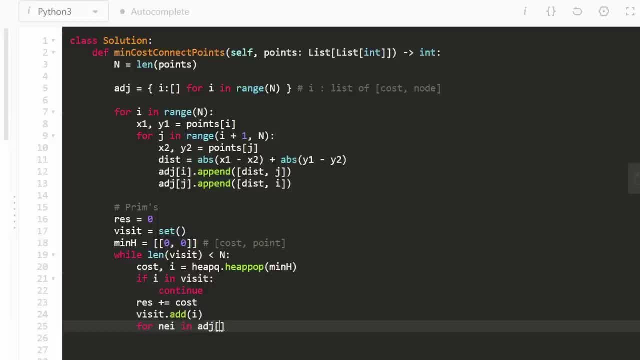 and then we're going to go through every neighbor in its adjacency list. so the adjacency list of i and remember each neighbor actually isn't just one value, it's going to be the cost- so let's call it neighbor cost- as well as the cost of the node. and then we're going to go through each neighbor in. 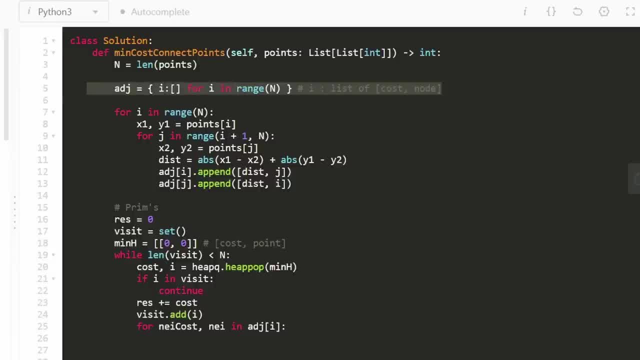 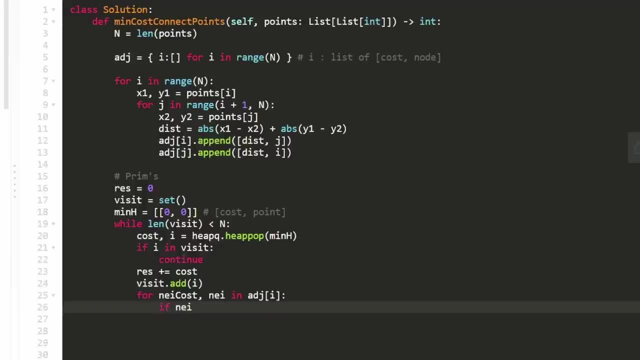 its adjacency list as well as the neighbor right up above. you remember that in our adjacency list we added a pair of values in that list: cost and the node itself. so now for each neighbor, so for ne. if the neighbor is not in visit, then we're going to be adding it to our min heap, so then we can say: 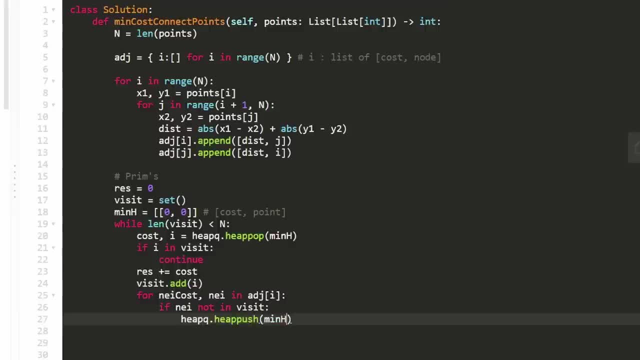 heap: q dot heap: push to the min heap. we're going to be pushing a pair of values. remember: we're pushing the cost first, so neighbor cost and then the neighbor, and that's it right. so we're just for every neighbor. all we're having to do is just add it to the min heap and then we're going to. 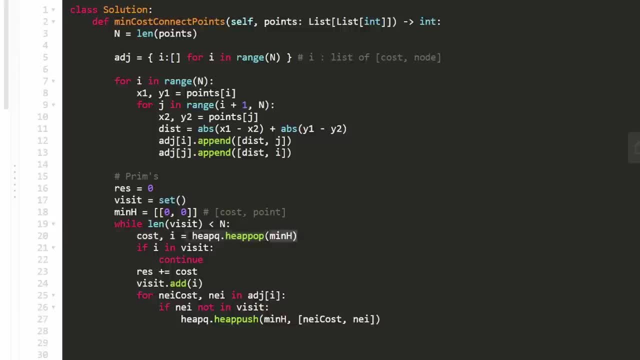 the min heap right, and then we're going to go to the next iteration of the loop, repeat the exact same thing until we visit every single node. once we've done that, we know for sure the result has the total cost that it took. so then at the end, all we have to do is return that cost. let me make sure.